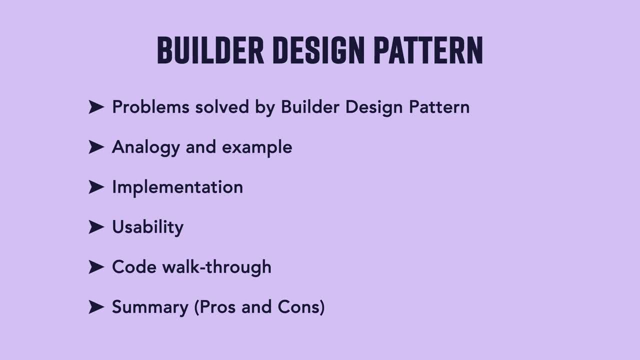 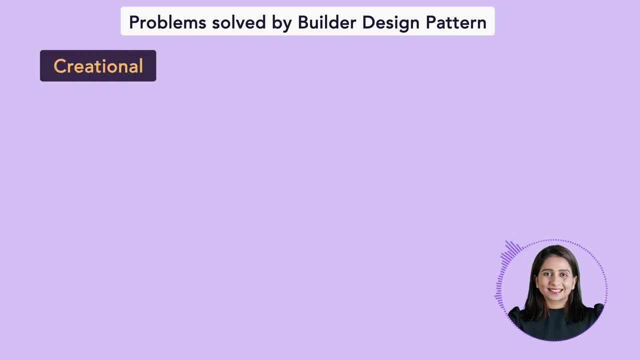 Followed by summary and pros and cons of builder pattern. So let's get started, Since builder pattern is a creational design pattern and it is utilized for creation of objects, But the problem that builder pattern specifically solves is creation of complex objects. Whenever there are scenarios which end up in classes which have complex constructors, builder pattern comes to rescue. One of the solutions for those complex constructors is telescoped constructors. 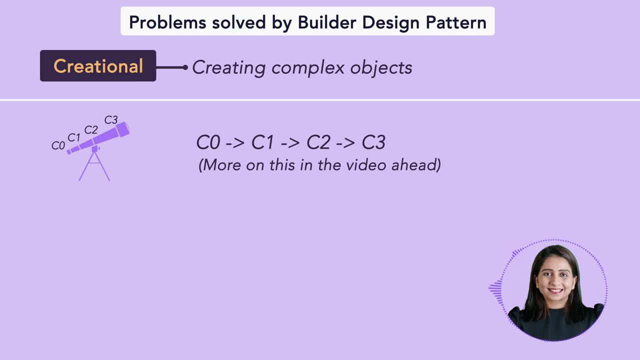 But again, telescoped constructors are not able to solve the problem in a way that builder pattern can solve. Builder pattern also helps with classes and objects which require the functionality of immutability, And also, once implementing the builder pattern, there is less need for exposing the setters of a class. We will see all of this in our code walkthrough of how these problems are solved using builder pattern, But before that, let's try to understand the concept and ideology behind the build pattern through an analogy. 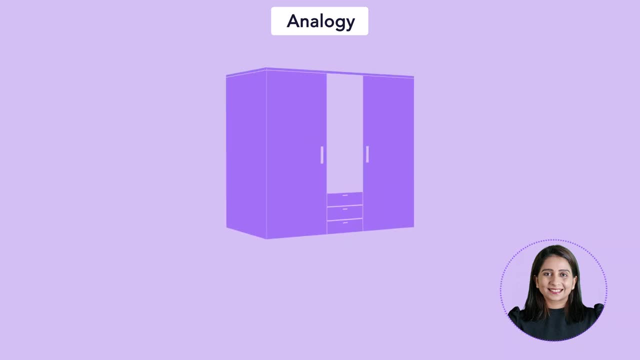 Let's consider a scenario of building a wardrobe. As you know, wardrobes can be of multiple types. They can have one door, two doors, multiple doors. There can or cannot be mirrors on the wardrobes. Also, the material of the wardrobe can be metal, wood, plastic or something else. There can be a feature of hanging rods in the wardrobes, and the number of compartments in a wardrobe can vary. 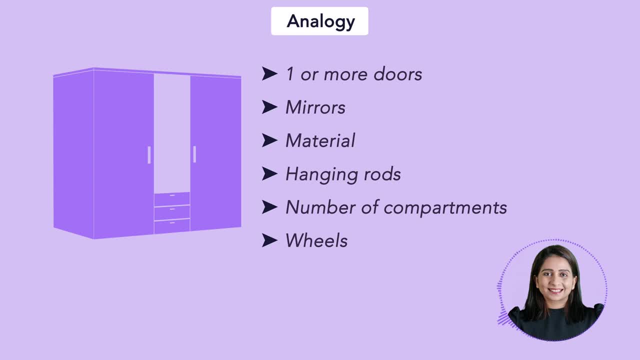 Some wardrobes might come with wheels as well. As you might have guessed by now, that is what building a wardrobe is: that some features in the wardrobes are going to be essential, like the doors and locks and so on, but some features, like the mirror on the wardrobe door or the wheels, might be optional for some. 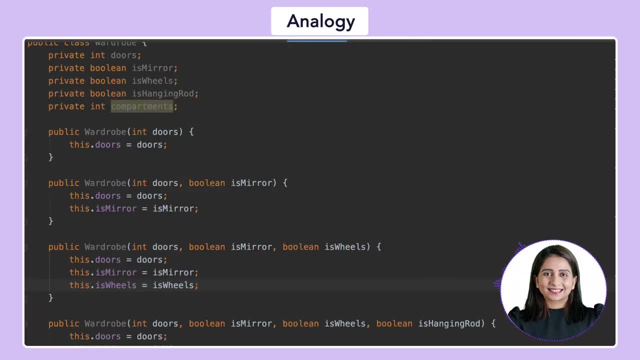 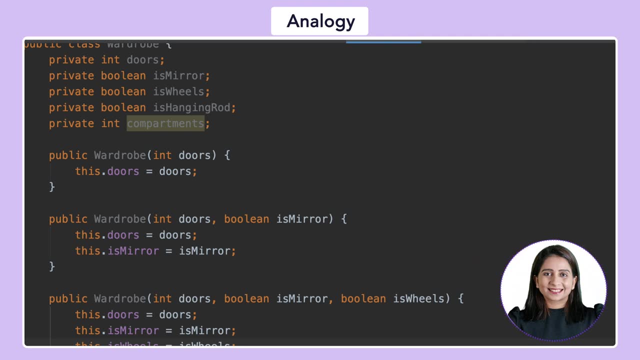 particular wardrobes. if we have to code it, then this is how the code is going to look like: there would be a class wardrobe with the fields as doors, mirror, hanging roads, compartments and wheels, and the constructor of the wardrobe would be something like this: one constructor would take 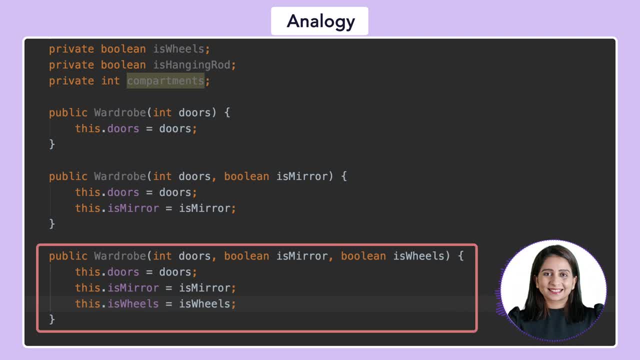 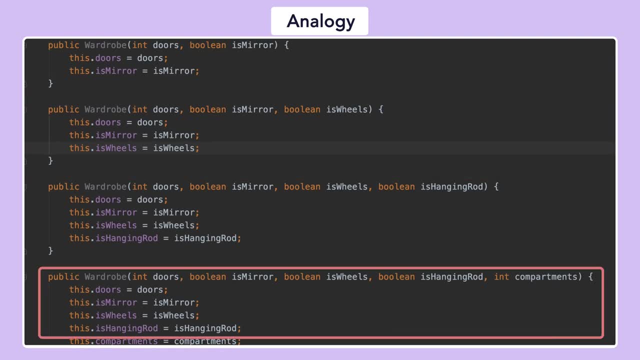 doors and mirror as parameters. another might take door, mirror and wheels. one might take door, mirror, wheels and compartments and there would be one constructor which take all the parameters. now this seems to be perfectly decent code and you might not see what's the problem with this code in. 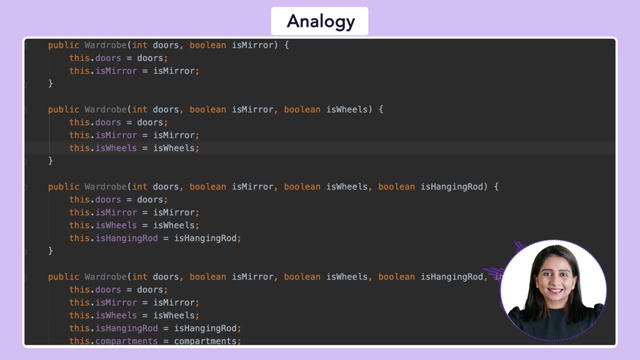 the first look. but here is the issue. let's say that you want to build a wardrobe which just has doors, mirrors and compartments. now there are two ways to go about it. either you create a constructor or you create the famous food. that's the question. and area goes on to build theiera. 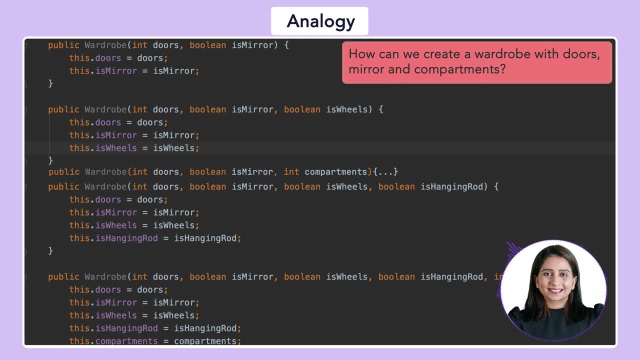 which has door, mirror and compartments, or you utilize this particular constructor over here, but the value for the hanging road and the wheels is going to be null. Think about the problems that would arise in the code if an extra field has to be added in this class. How many permutations and 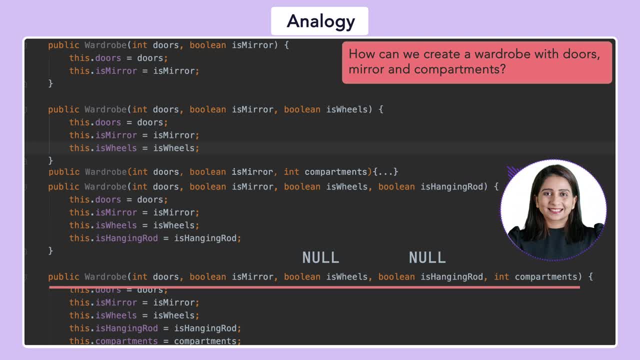 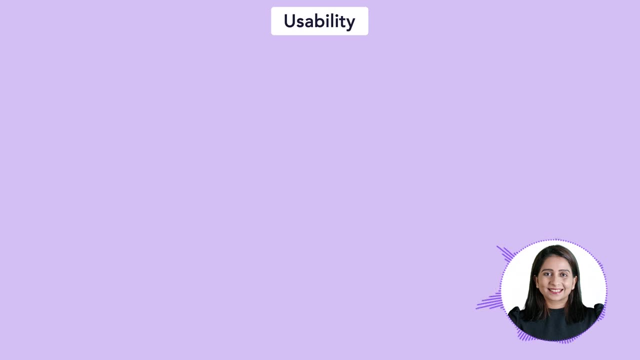 combinations you would have to manage in order to create those constructors. We will see how builder pattern solves the problem of complex constructors as well as telescoped constructors, but before that, let's first try to understand what's the difference between implementing a builder pattern versus using a builder pattern. I am sure many of you must have. 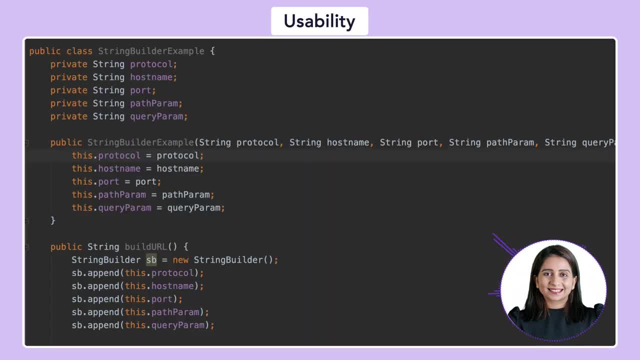 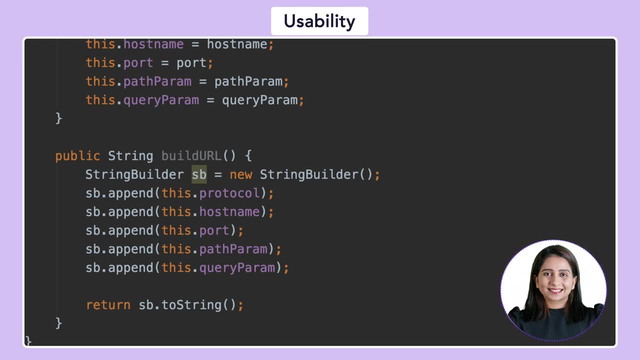 already utilized java's string builder functionality, where you just initialize the string builder and keep appending the strings onto the builder and finally call sbbuildtrueString. Now this is the utilization of a builder pattern, because string builder is a builder class which helps you to concatenate strings one after the other and finally returns you a string which you cannot change. 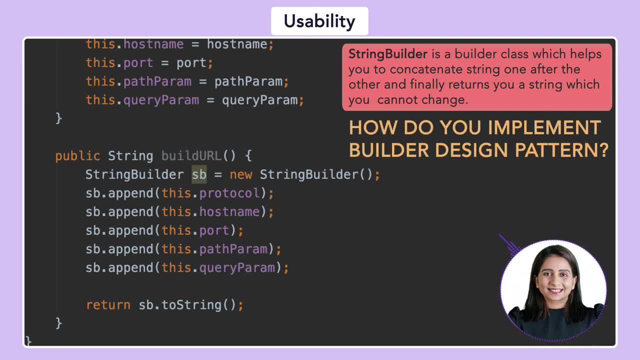 This is how you utilize builder pattern. But if you want to use a builder pattern, you need to use a string builder. But how do you implement the builder pattern if you have to build something yourself or if there is a use case that you are working on which requires the implementation of builder pattern? 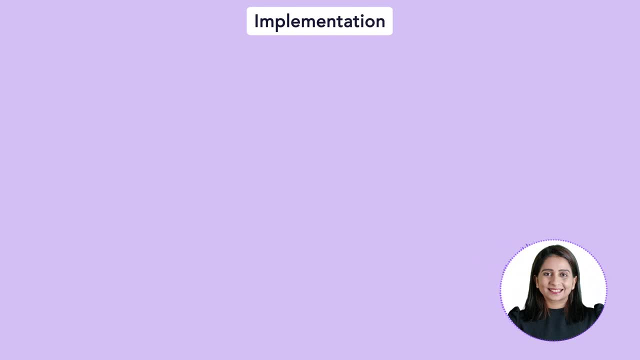 In order to understand the implementation of builder pattern, we will take example of URL builder. Let's try to understand how to implement builder pattern. Let's say that we have to implement a URL builder, which allows us to form a URL given some parameters. Now, as you know that a URL is composed of protocols, protocols and parameters. 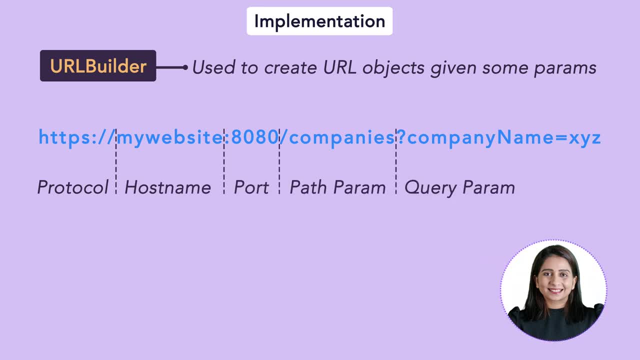 You can see that we have the protocol, hostname, port, pathparam and queryparam. Now you might also know that every URL would need protocol and hostname, but every URL might not need port, it might not need pathparam or it might not need queryparam. All these three parameters are 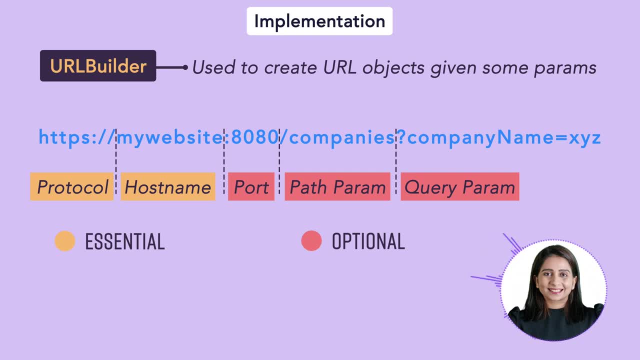 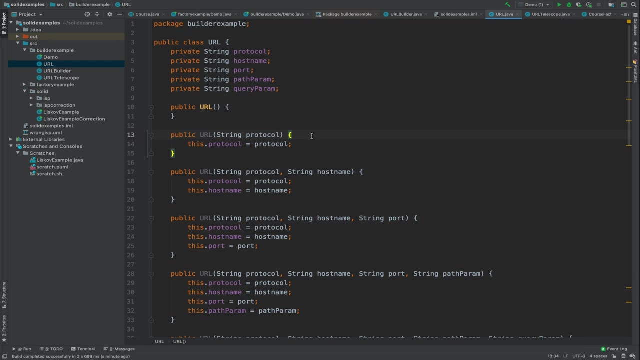 optional, So you can see the different combinations here that you would need if you go with normal constructor method. Now let's dig deep in the code and understand how we can solve this using builder pattern. Let's try to understand from the code how we can use the builder design pattern to create a URL builder class As. 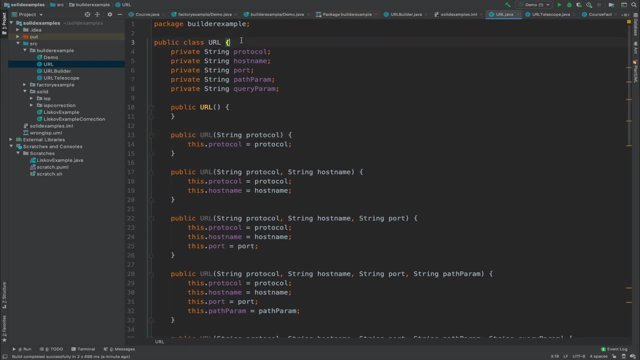 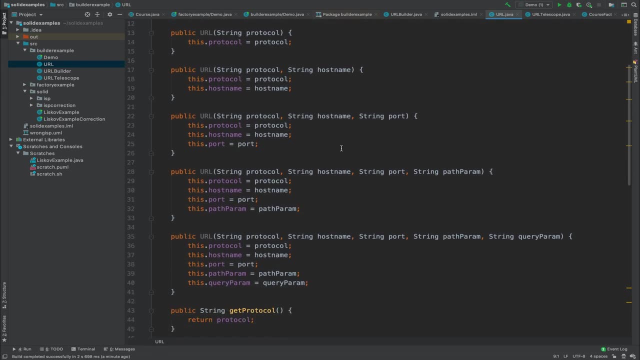 you can see over here that there is a URL class over here which has certain fields added to it, and then there are certain constructors which take one, two or three parameters or here in this case, even four parameters, to create an instance of this URL class. There are also different getters and setters. 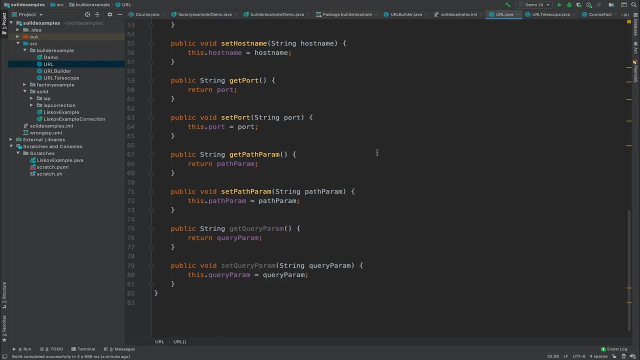 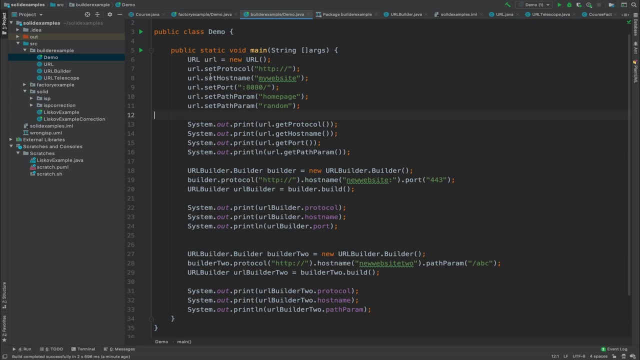 provided here, and this is just for the example. you can have either of them. you do not need both the setters as well as the constructors. Now let's say in the demo class how the object of URL class is created. This is how we instantiate the URL object. you can also use one of the constructors with the set fields. 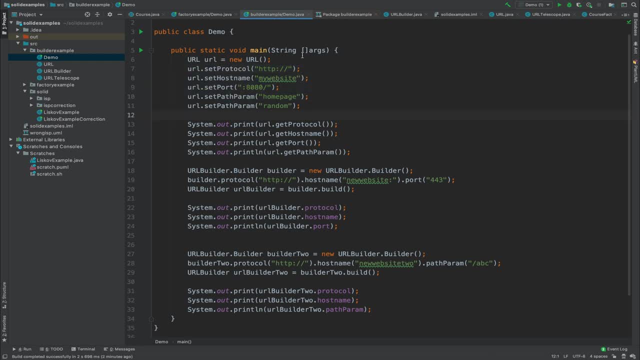 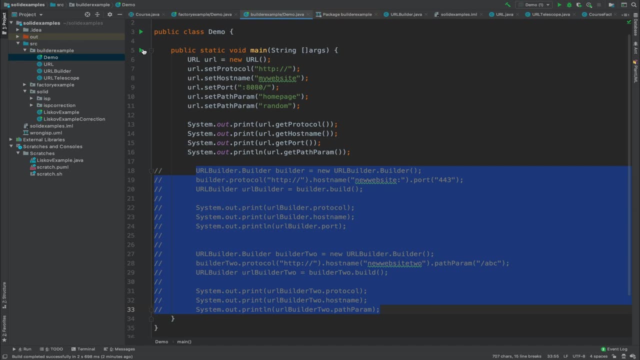 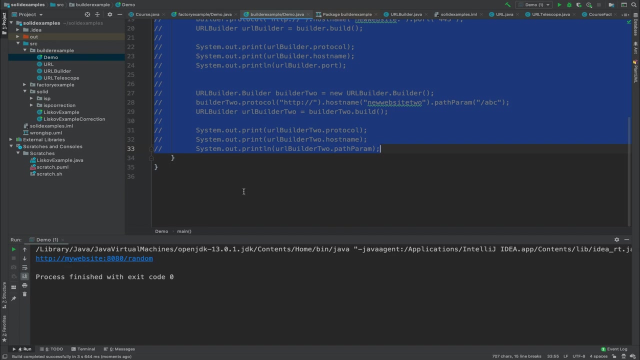 here I am using the setters. Once we instantiate this object and set all the fields, we can see how this code runs. but before doing that, let me just uncomment this builder code over here and let's try to run only this part. As you can see, we have the whole value of URL over here. Now let's go back to the. 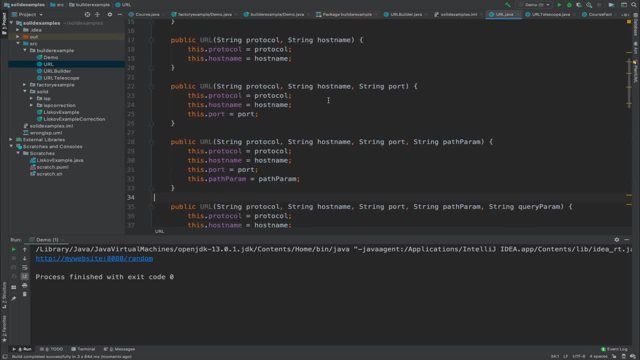 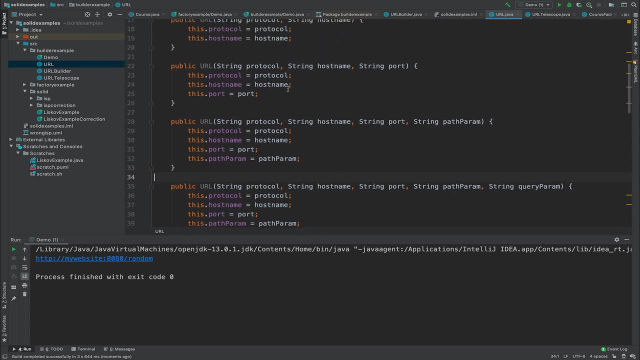 URL class and see what's the issue is, As you can see, that there are a number of parameters and hence we have to create a lot of constructors. Now, what happens? if there is a case when you have to have a constructor which accepts protocol, host name and only path params, then you would 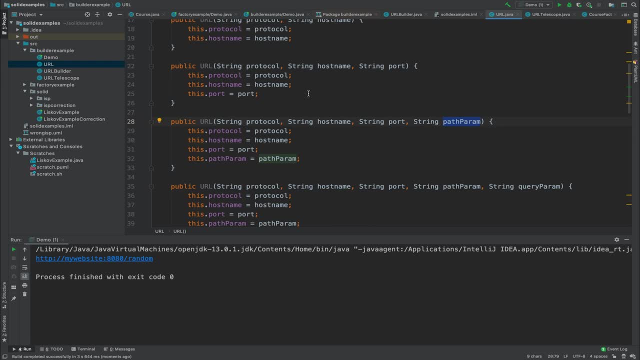 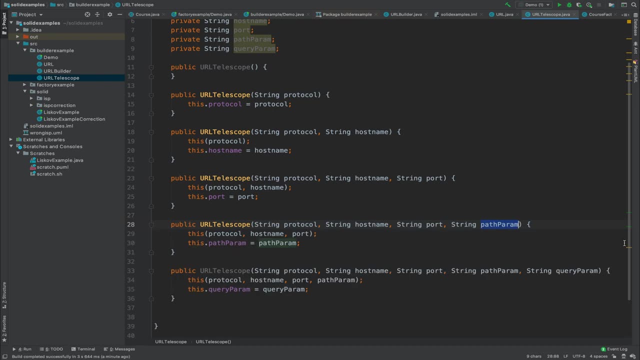 need to create a third constructor, and this would just add a lot of lines to your already lengthy code. One problem to solve this is the telescoping constructors, and here is how telescoping constructors work: Instead of initializing a lot of constructors, one constructor utilizes the already initialized. 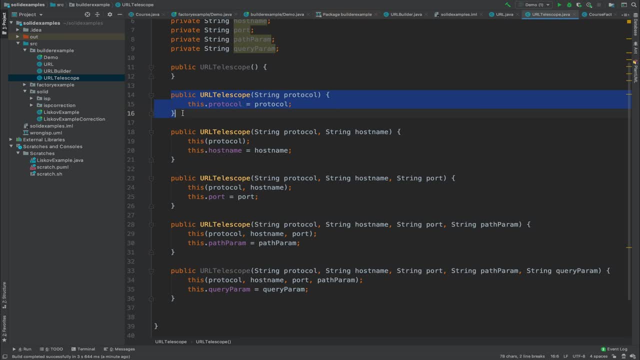 constructor, as you can see here that we have this constructor over here which has protocol parameter, the another constructor, which has protocol and host name, utilizes the first constructor, the third constructor over here utilizes this constructor, and so on and so forth. this way of coding solves one problem. 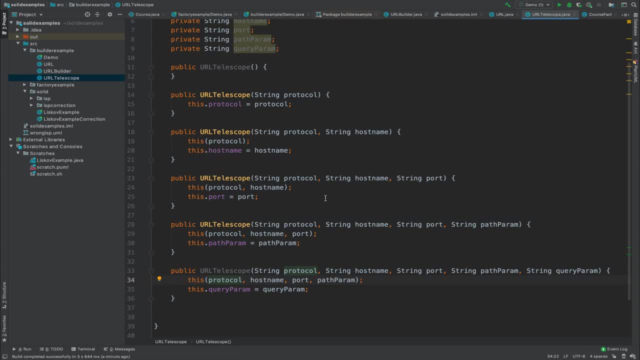 that your code becomes less lengthy, but again it does not solve the problem of having multiple combinations. let's say again the same example: that you need a constructor which requires protocol host name and path param. in that case you would have to write another constructor and thus telescope constructors do not. 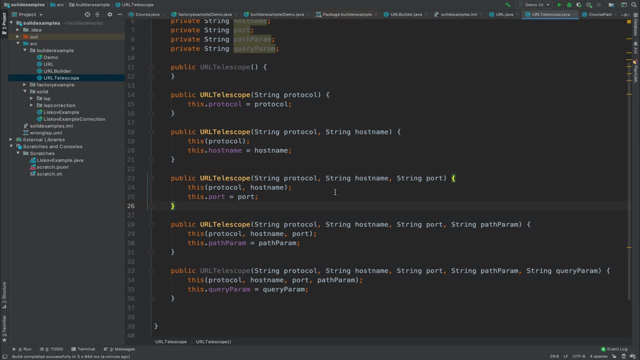 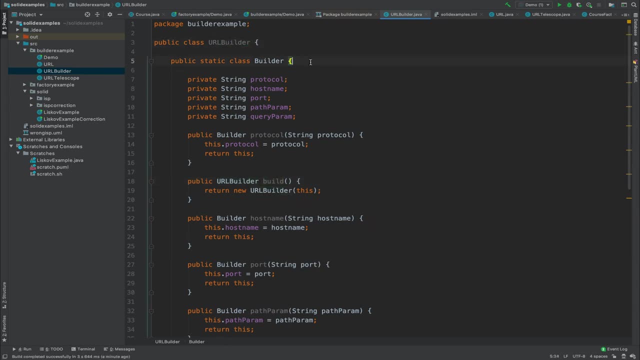 solve the problem hundred percent. here is when the builder pattern comes into the picture. let's look at the class URL builder- how we will solve it using the builder pattern. for builder pattern you need to have an inner static class called builder. it has the same fields that. 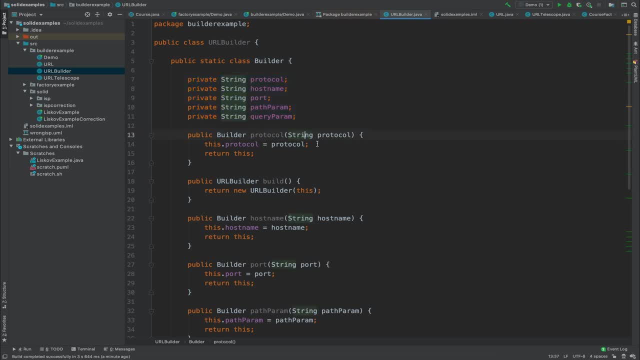 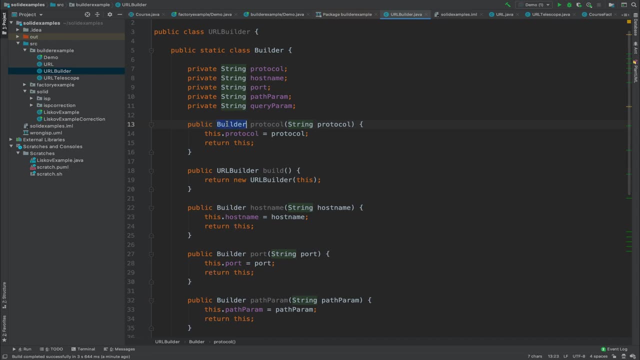 the base class has to have. apart from these fields, it has constructors for all these fields, with the only exception that it returns the builder type. it returns the instance of the builder, builder class, instead of returning anything else, so that this particular instance of this particular object can. 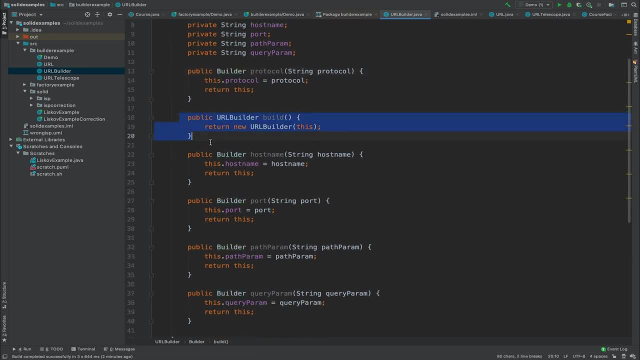 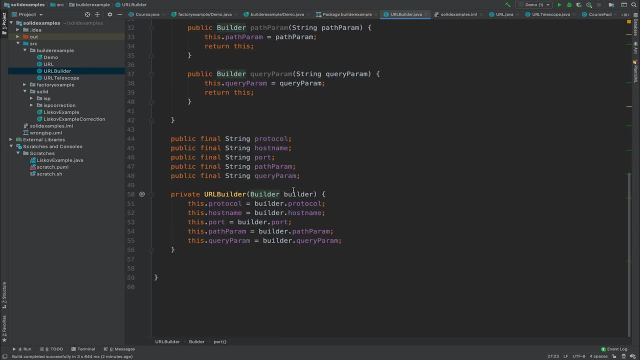 be plugged into this particular URL builder class and you can get the instance of URL builder class itself. finally, in the URL builder class you can see that the instance of builder is passed on and it helps to set value of different fields. as you can see, here it's pretty clear that you can add more. 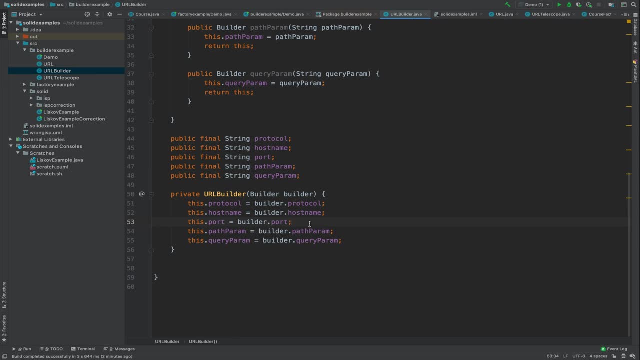 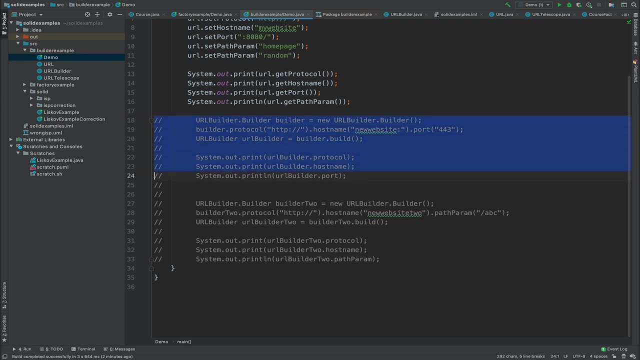 parameters. here you can remove any parameters if you need. now let's move on to see how this is actually utilized, and in order to do that I would have to comment the code. and let me comment the code only till here, to show you the first example. in this first example, we have first created an object of the builder. 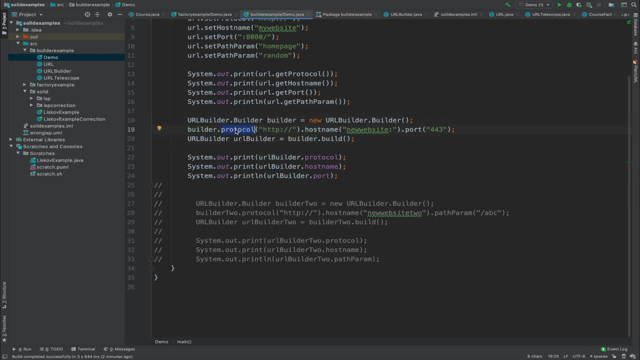 class and then we are calling the constructor of those builder class and builder classes like builderprotocol and we supply the value hostname. why this chaining is possible? because protocol is returning this object itself, on which you can again call host name and on the top of which you can call port. finally, you call this function builderbuild. 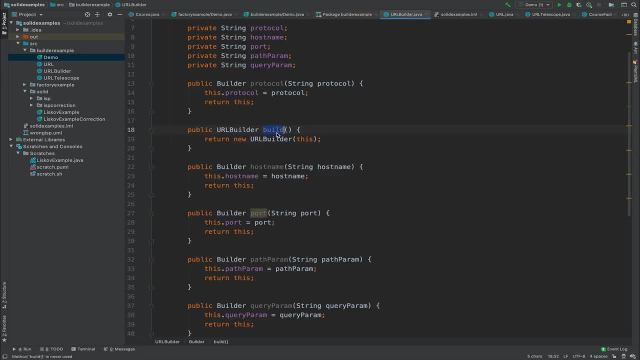 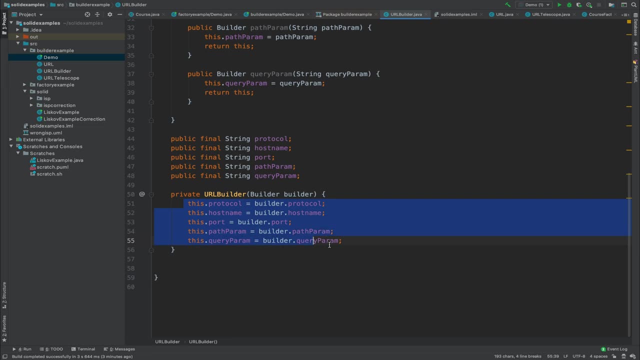 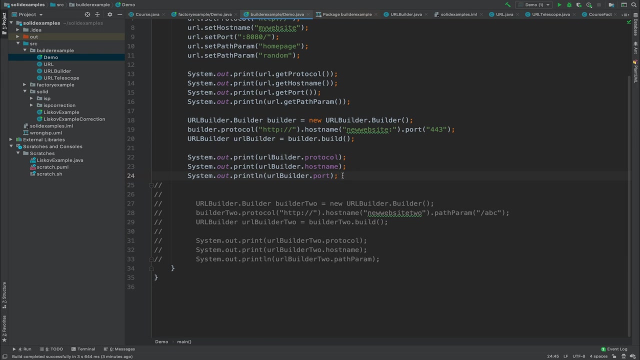 let's see what this particular function does. this particular function calls the url builder class with the builder object itself which, again, as i showed you before, sets all these fields. now, if we go back to our demo and try to run this particular function, which just prints out all these value, 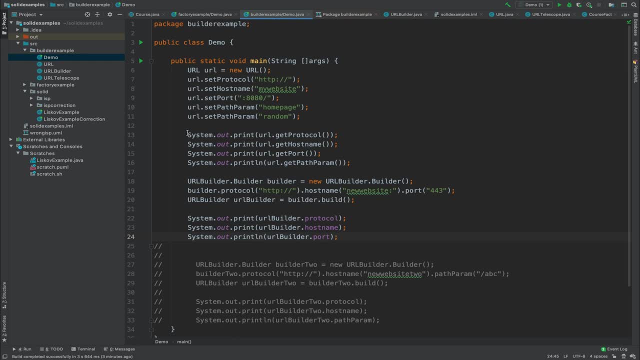 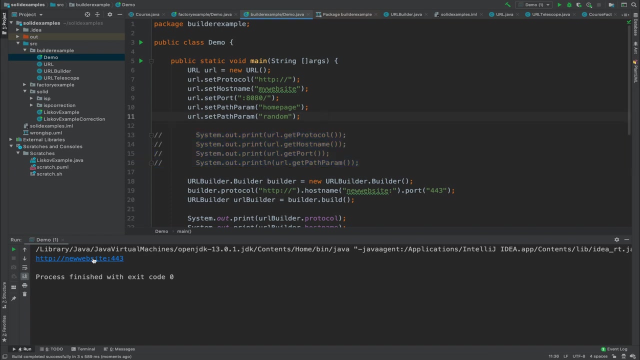 let's see what happens. before doing that, let me comment out this code so it doesn't create any confusion. just like the previous class, which was vanilla, vanilla, java or with it was not using any design pattern, we have the whole code here using the builder pattern. you have your protocol host. 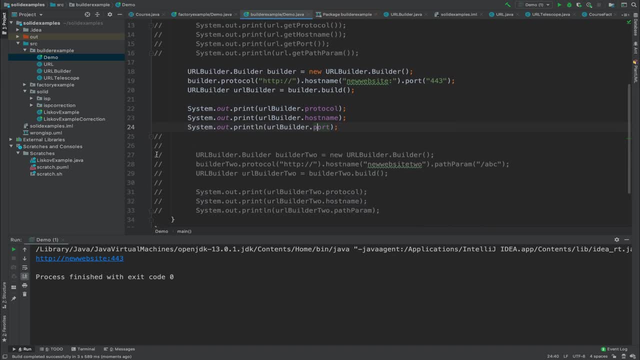 name and port. now, in case that you want to run this particular function, you can run this particular function which run the test. and if we want to run this program onida, you want a particular url which requires path parameter but does not require any port. what you can do in that scenario is you can. 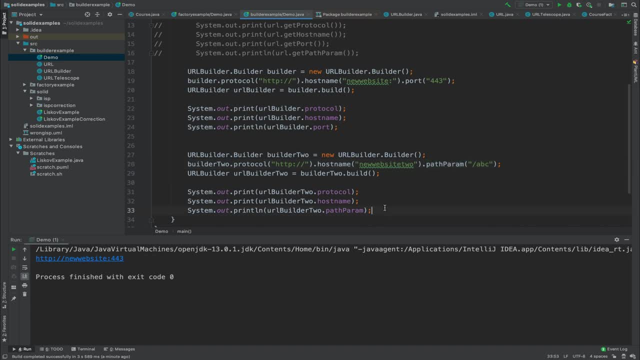 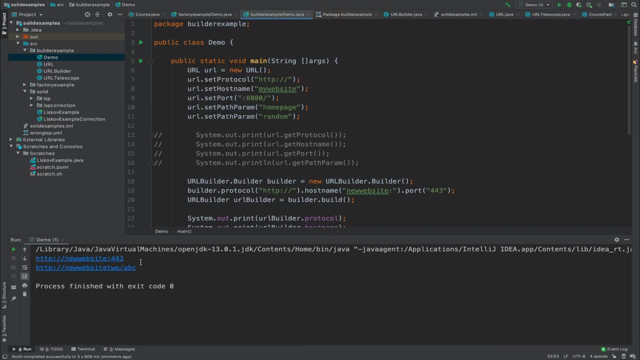 call builder to that protocol host name and only pathitter. you can completely skipport and it won't create a difference to your code. let's try to run this nc. as you can see here very clearly, we have our another url which has a path term, but but which? 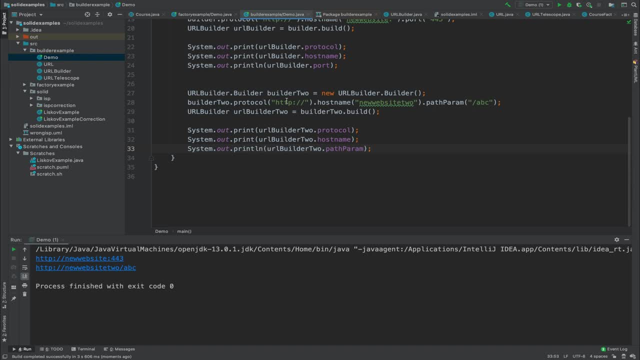 you can create any kind of URLs you want with any combination of necessary as well as optional features. So this is how builder pattern solves the problem of complex constructors, as well as on classes which have multiple parameters and do not require all of them to create objects. 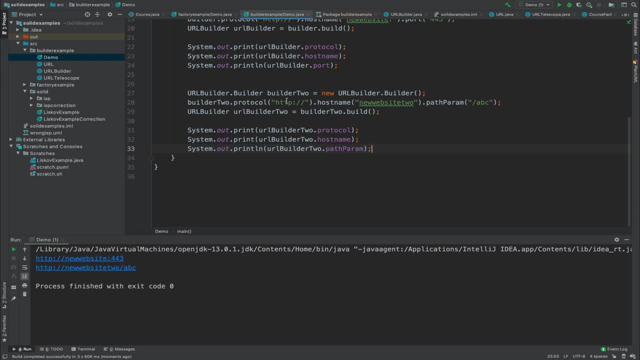 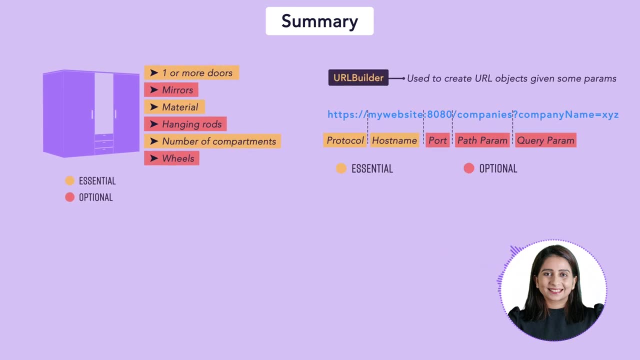 I hope this makes things further clear for you. Now let's go back to the summary. I'm sure that after going through the two examples of wardrobe and URL builder, you would be able to understand how builder pattern is utilized and how it solves problems of having complex constructors and 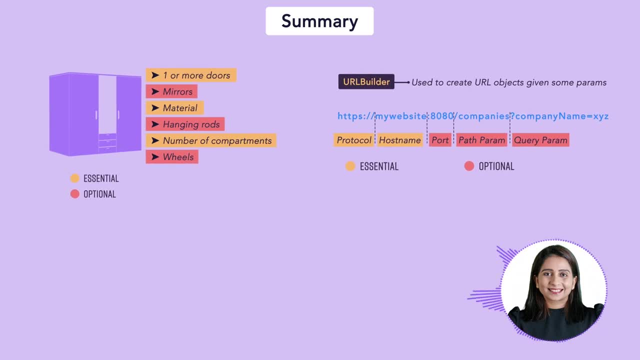 constructors which might have a lot of parameters. Let's try to summarize what we have learned today. There are some pros of using builder pattern. It is a good way to handle complexity and complex constructors. It is relatively easy to implement than other patterns. You just have to use an. 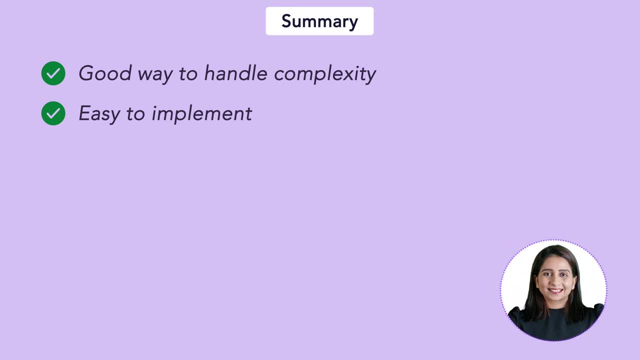 inner static class, typically in a java implementation, and this is a pattern that you can refactor your code later into. This is not a pattern that you can refactor later into. It is a pattern that you have to start implementing from the scratch. However, there are some cons as well, For example, 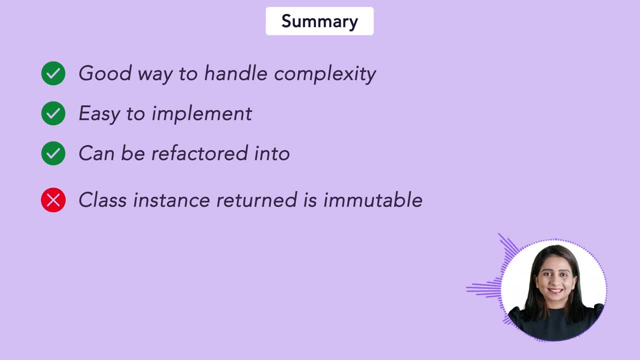 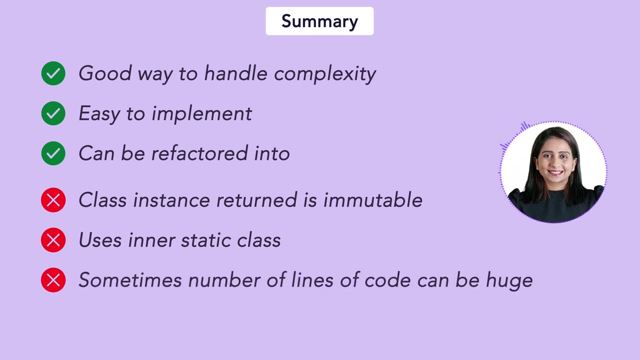 the class instance written by the builder pattern is immutable, so you cannot make any changes to that object. Also, it uses an inner static class for implementation, which might seem confusing to some folks. Sometimes the number of lines of code that you have to write can become huge in order to 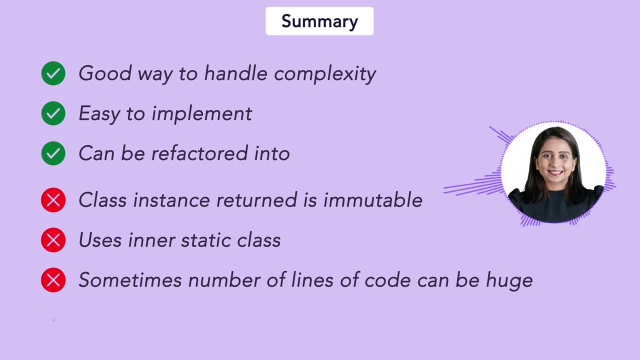 implement a builder pattern, although it is not that complex. Also, whenever you are using builder pattern or refactoring your code into a new one, it is not that easy to implement a builder pattern. You have to think of end-to-end use cases, So you have to think of design. It is not a con per se, but 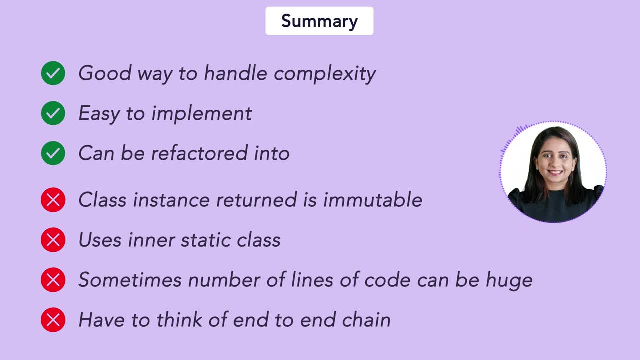 this is a factor that you have to take into account while implementing the builder pattern. I am sure after watching this video, it must be clear to you what is a builder pattern, how you can utilize a builder pattern and how you can implement your own builder pattern if there is a 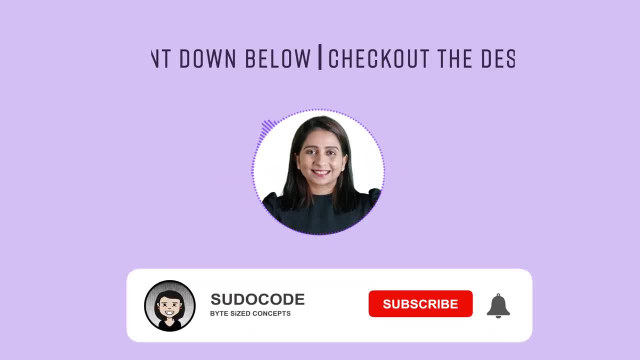 use case in your work to do so. If I have left out anything, or if you have any doubts or comments, please feel free to leave them in the comment section and I will try my best to get to them. Till then, take care, see you in the next video. Bye.